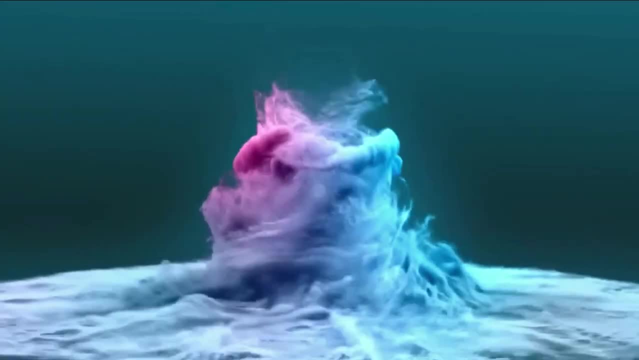 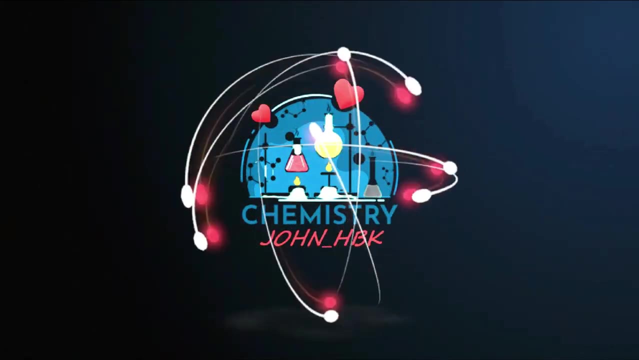 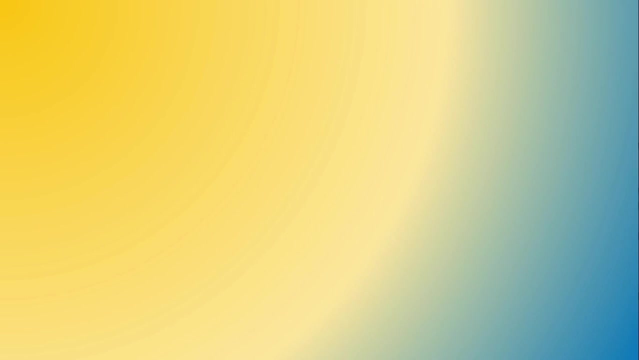 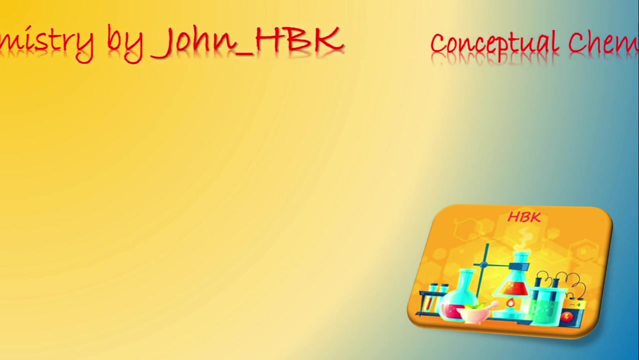 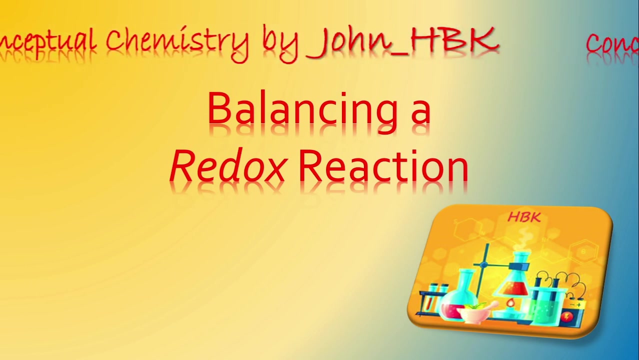 Hello guys, welcome to my channel. conceptual chemistry demystified by John HBK. Today, let's demystify balancing a redox reaction. Before continuing with the video, I would strongly recommend you to see my previous video on redox reaction basics. It will be helpful. 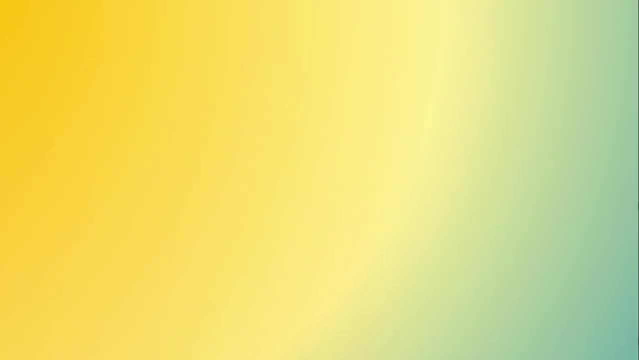 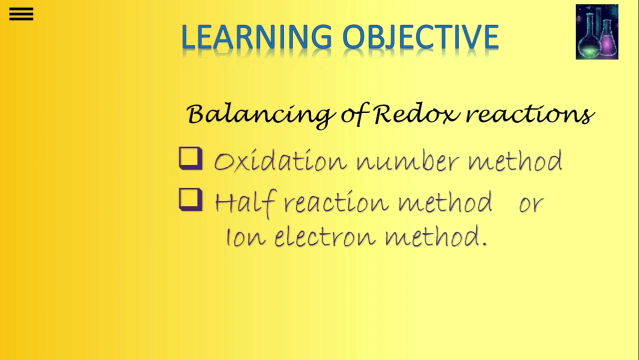 in understanding the following lecture. Let's look into our learning objective: Balancing of redox reaction by the following methods: Oxidation number method and half reaction method or ion electron method. So let's see what is oxidation number method, Oxidation. 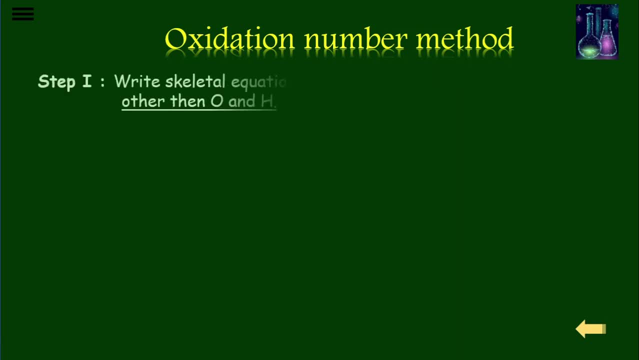 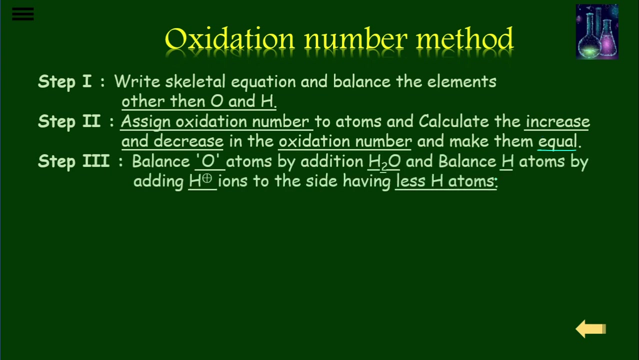 number method involves the following steps: Step 1, write skeletal equation and balance the elements other than oxygen and hydrogen. Step 2, assign oxidation number to atoms and calculate the increase and decrease in the oxidation number And make them equal. Step 3, balance oxygen atoms by adding water and balance hydrogen. 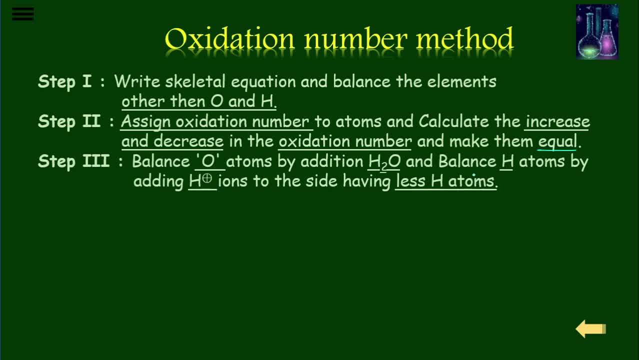 atoms by adding H plus ion to the side having less hydrogen atom. Step 4,: if the reaction occurs in basic medium, then add OH minus ions equal to the number of H plus ions in step 3 on both the sides of the equation, And step 5.. 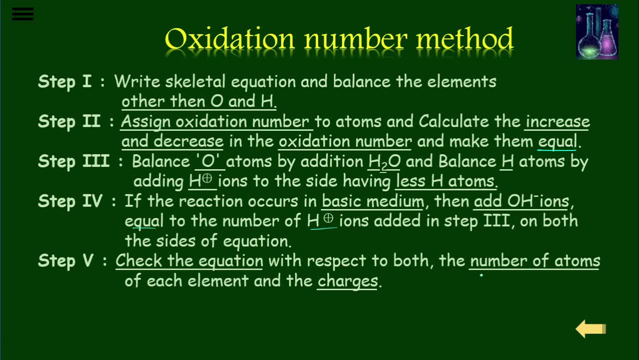 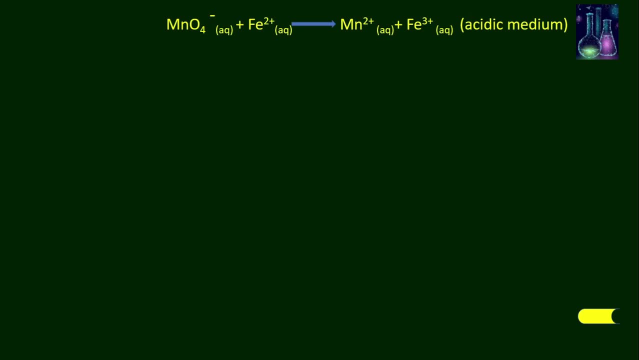 Check the equation with respect to both the number of atoms of each element and the charges. So now let's move on to an example and apply these steps to balance a redox reaction. Now we have a skeletal equation in front of us. Let's assign the oxidation number to: 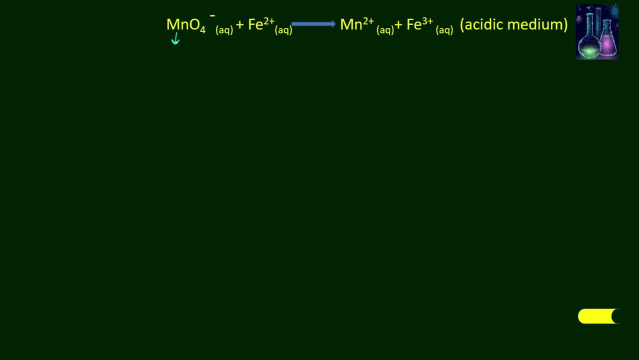 each of the elements Manganese here shows plus 7. Oxygen minus 2. Fe plus 2.. Mn plus 2. Fe plus 3.. So we have assigned the oxidation state, and now let's see the increase and decrease in. 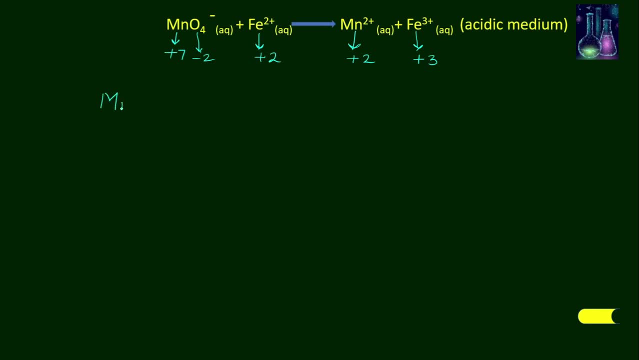 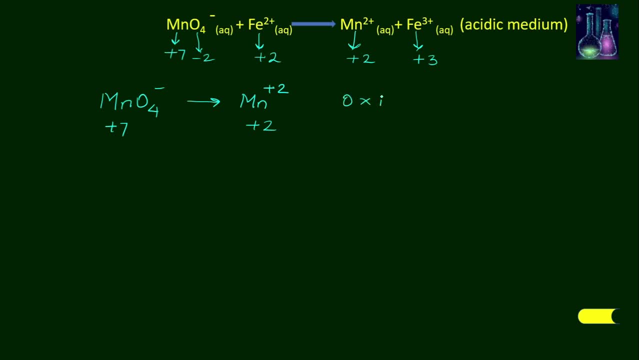 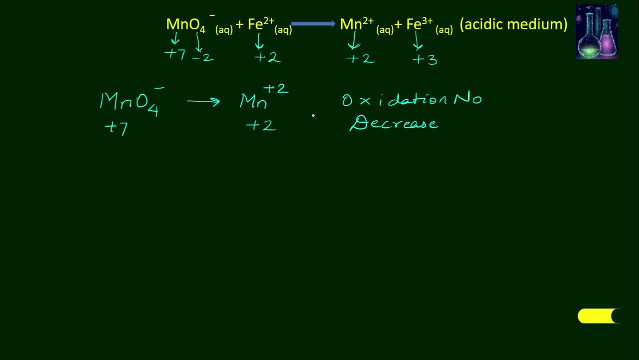 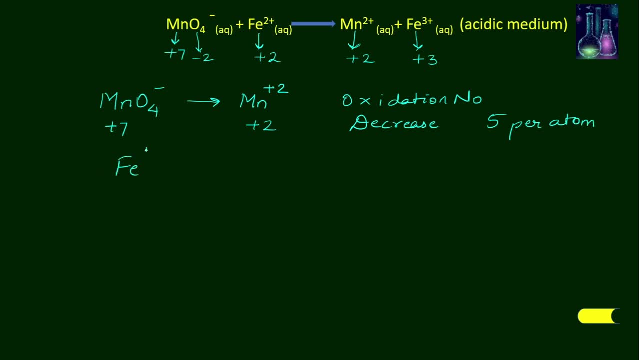 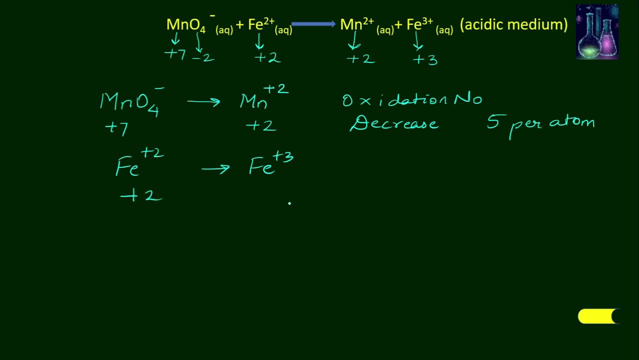 Fe plus 3.. Further, the oxidation number increases from plus 2 to plus 3, that is, by one Increase by 1 per atom. so therefore, to make it equal, I have to multiply this by 5.. Now write the equation: MnO4 minus plus 5 Fe2 지. 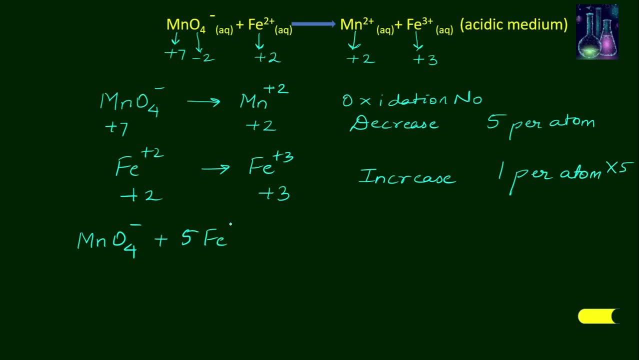 Qθ enjoyed Fe plus 2 plus, gives Mn plus 2 plus 5 Fe plus 3.. Now here the oxygen is not balanced. Now the atoms are balanced, but oxygen is not balanced. So to balance oxygen we put water. on the opposite, 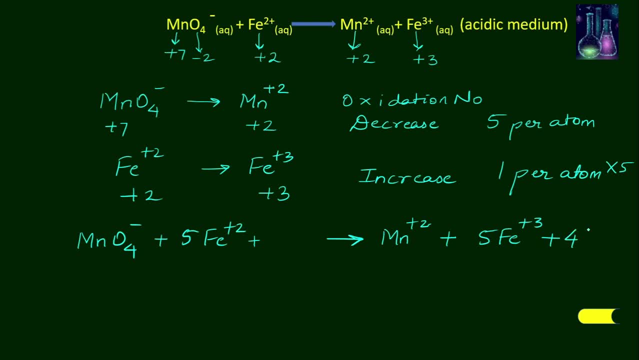 side of the equation, There are 4.. So here there are 4 water molecules that we added, and when you are putting water there are 8 hydrogen atoms. Since the reaction is an acidic medium, we will put 8 H plus ions. So now let's check whether the reaction is balanced. 1 Mn. 1 Mn- 4 oxygen. 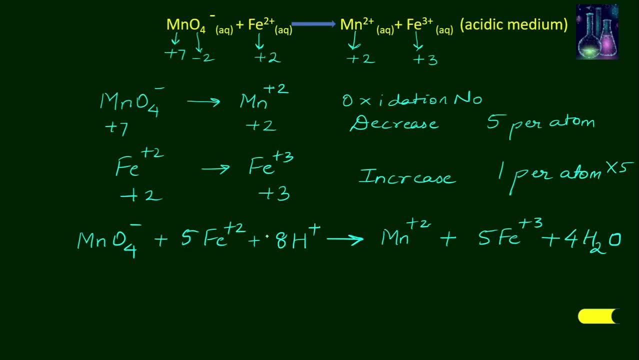 4 oxygen: 5 Fe, 5 Fe. 8 hydrogen, 8 hydrogen. So the atoms are balanced. Now what about the charge? Let's check out Minus 1 plus 5: 2 is a 10, plus 8: 1 is a 8.. This makes up a total. 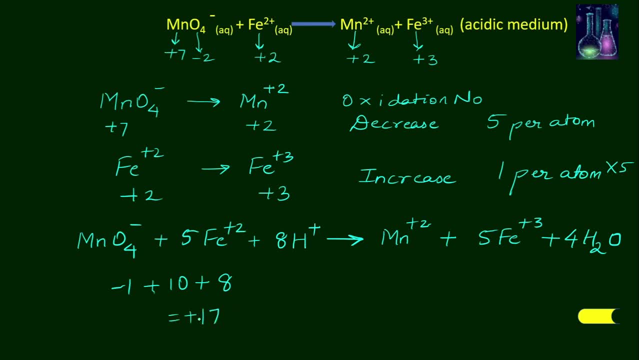 charge of 17.. Plus 17.. And here, plus 2 plus 5, 3 is a 15. plus water is a neutral molecule. Therefore the overall charge is plus 70.. Now we have the charges also balanced, as well as the atoms Now. 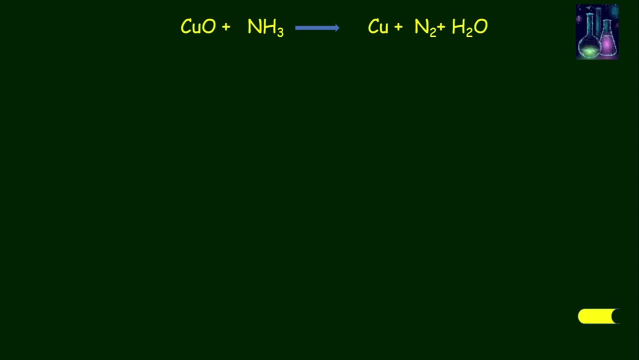 let's move on to our next example. First we have the skeletal equation in front of us. Let's balance the atoms other than hydrogen and oxygen, So 1 copper, 1 copper. 2 nitrogen, 1 nitrogen. So I'll put 2 here, Then assign the. 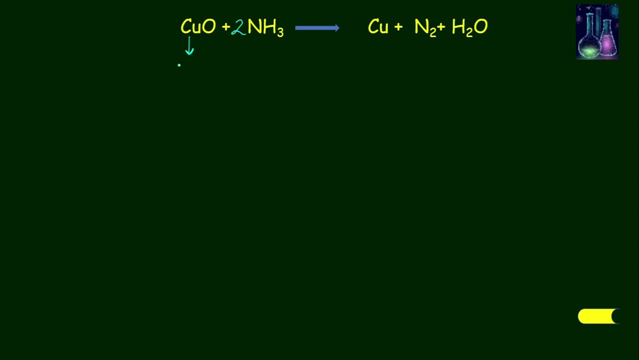 oxidation numbers: Here copper is plus 2. Here oxygen is minus 2. Nitrogen here is minus 3. Hydrogen here is minus 2. Nitrogen here is minus 3. Hydrogen here is minus 3. Hydrogen here is minus. 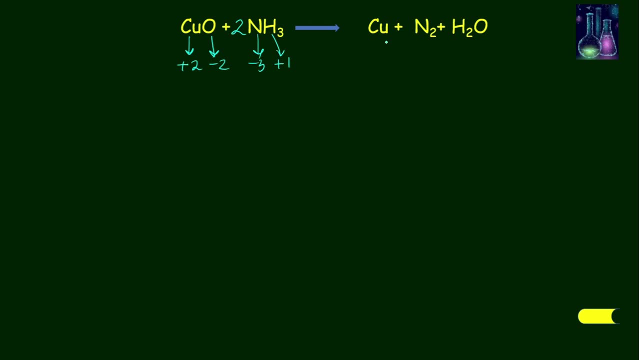 3. Hydrogen: here is plus 1.. Copper in free state: 0.. Nitrogen in free state combined with itself: 0.. Hydrogen plus 1.. And oxygen minus 2.. Now let's see the increase and decrease in oxidation state. 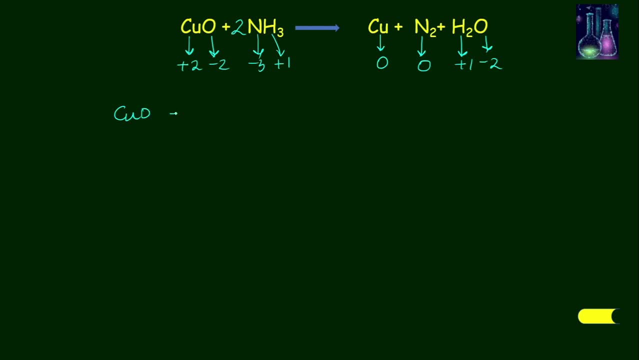 per atom. In the case of copper oxide to copper, the oxidation state changed from 1 to 2.. So this is changed from 0 plus 2 to 0. That is decrease of 2 per atom. In the case of ammonia, NH3 to. 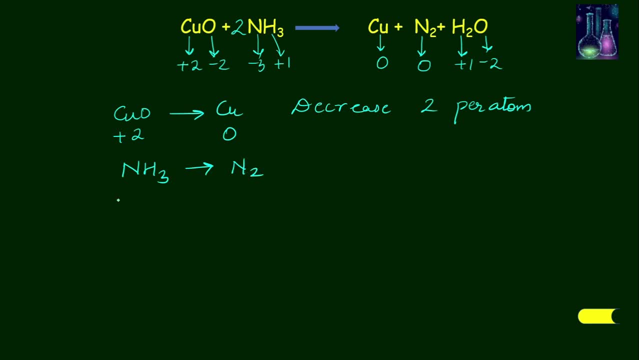 nitrogen. the oxidation changed from minus 3 to 0. That is it increased by 3 per atom. Therefore we have to make this multiplied by 3, this multiplied by 2 to make it equal. So we will write the equation: 3 CuO plus. we have already multiplied here 2.. So 2 NH3 gives 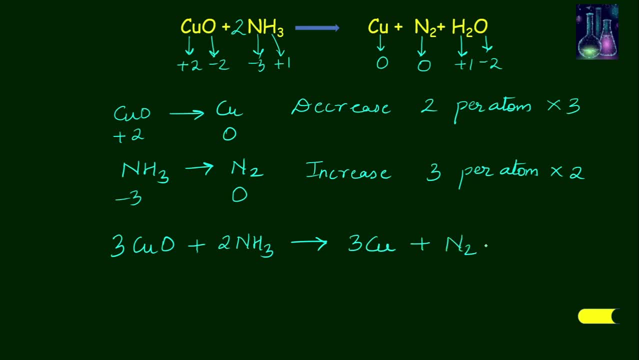 3: CuO Plus N2 plus H2O. Now let's see the atoms copper and nitrogen balanced. Now let's balance oxygen. There are 3 oxygen over here and there is only 1. So to make it 3, I multiplied this by 3.. 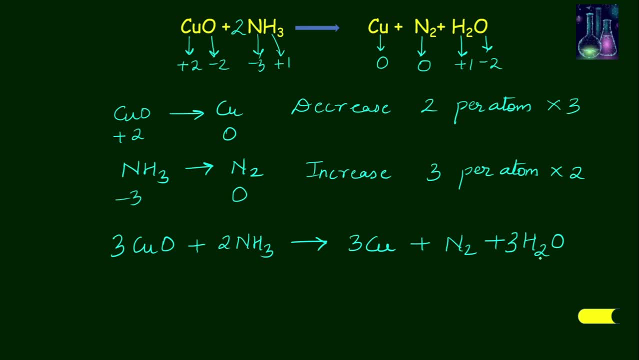 3 oxygen. This makes up 6 hydrogen, 3 to the 6, and here I have 3 to the 6.. So 4 hydrogen is also balanced, And since all are neutral molecule, the charge also is balanced. Let's move on to our next example. So in our third example let's we have the skeletal equation in. 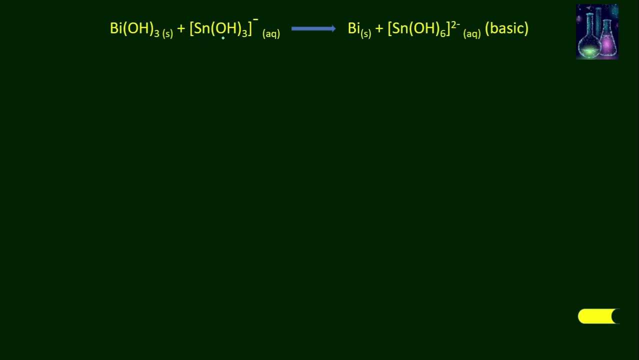 front of us Bismuth hydroxide reacting with the tin complex, giving Bismuth plus tin hydroxide complex. Now let's assign the oxidation number. Here Bismuth is plus 3. Oxygen minus 2. Hydrogen plus 1.. Here tin is plus 2. Oxygen minus 2. Hydrogen plus 1.. 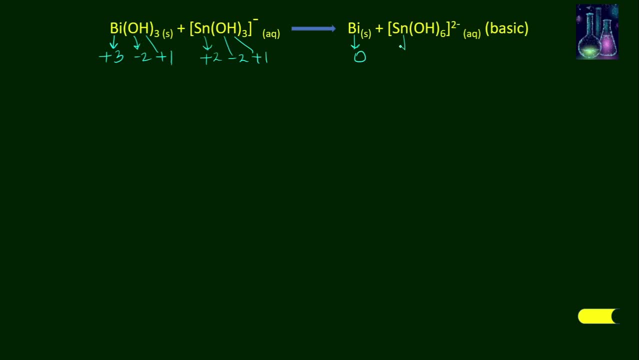 Bismuth here is single, Therefore 0.. Tin here is plus 4.. Oxygen here is minus 2.. And hydrogen here is plus 1.. And the reaction takes place in basic medium, Basic medium. Now let's see the increase and decrease in oxidation number. 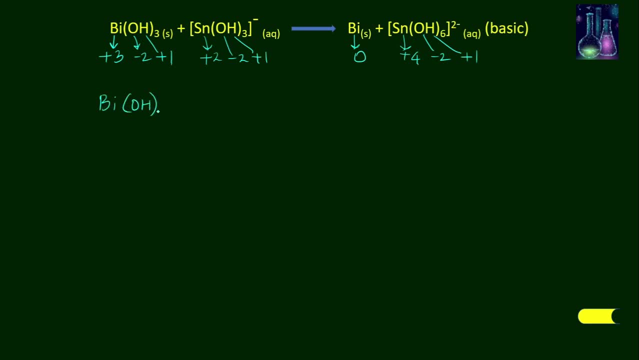 BiOH thrice converts into Bi And the increase, the decrease in oxidation number is from 0,, from 3 to 0. Therefore, decrease decrease by 3. And in the case of SnOH, the whole 3, overall charge minus 1, gives SnOH the whole 6, overall charge minus 2.. 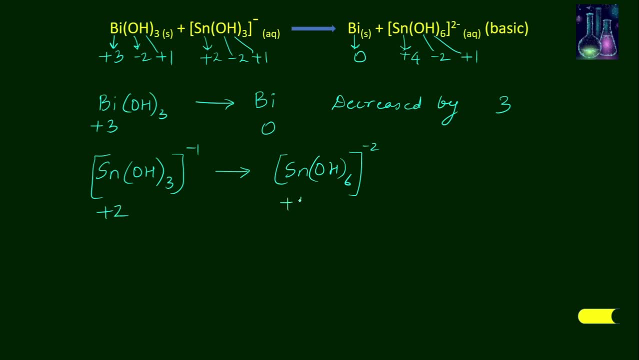 The change is from plus 2 to plus 4.. That means it is increased, increased by 2. Therefore, to make it equal, I have to multiply this by 2 and this by 3.. And therefore the reaction becomes 2: BiOH: the whole 3, plus 3. SnOH: the whole 3, overall minus 1,. 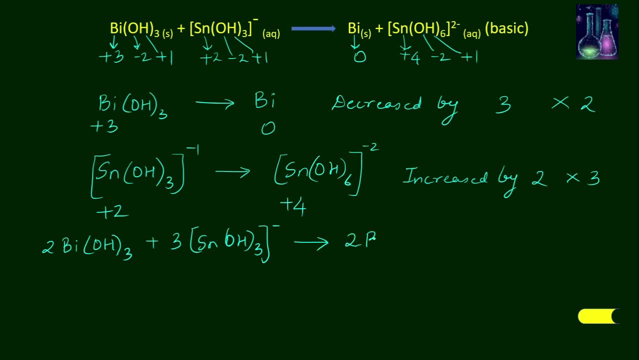 gives 2 Bi plus 3 SnOH, the whole 6.. The overall charge minus 2.. Now see, our atoms are balanced. Now let's balance oxygen and hydrogen. To balance oxygen we need to add water. Let's see how many oxygens are there. 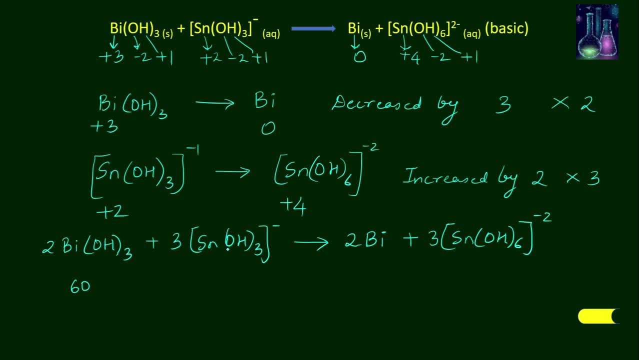 3. twos are 6 oxygens over here And 3. threes are 9 oxygens. So there are 15 oxygen molecules over here And here we have 6. threes are 18 oxygen molecules. So let's add water molecule to the. 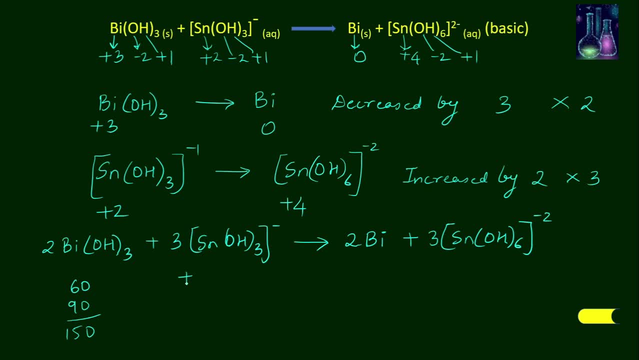 having less number of oxygen. so here I will add three molecules of water. this will make up 18. next see the molecules of hydrogen: 3 to the 6 hydrogen, 3, threes are 9 hydrogen and 3 to the 6 hydrogen. this makes up 15 and 6 makes up 21. 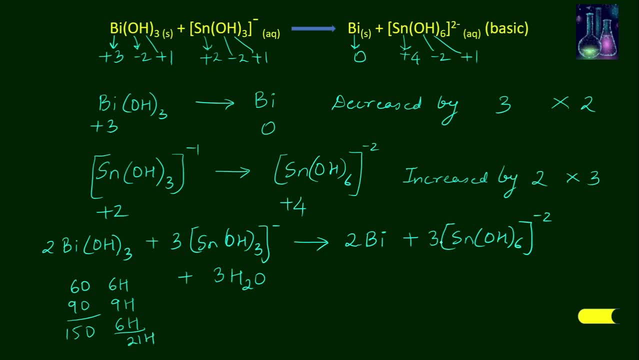 in one hydrogen. here I have six, threes are 18 hydrogen, now 18. so I have to add 3 H plus ions over here to make it balanced. but since the reaction is in basic medium, thus fourth step says that, or add OH ions equal to the number of H plus ions on both the sides of the reaction. so I will add. 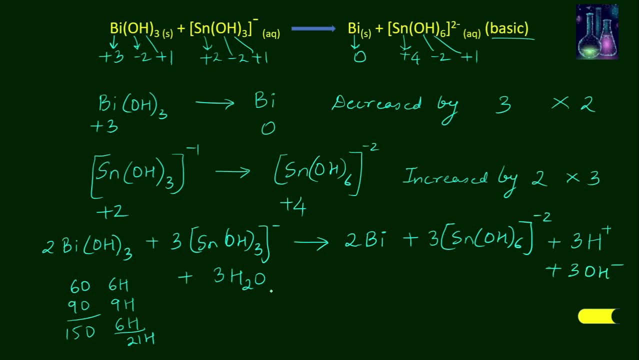 Here € 3 OH ions and here 3 OH ions and therefore I have the reaction in basic medium. Now this 3 H plus and this 3 OH will convert into 3 molecules of water and I can cancel that out and this 3. 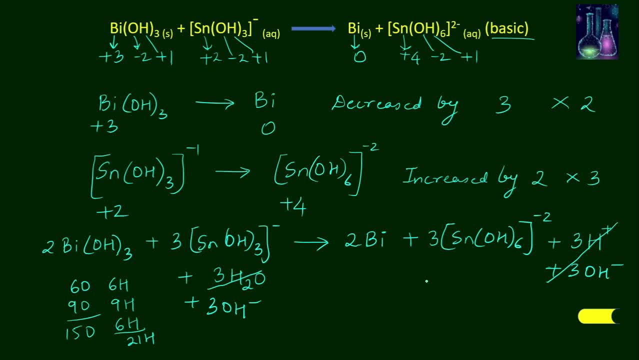 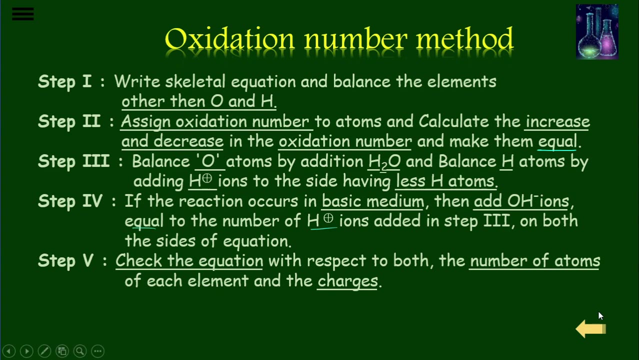 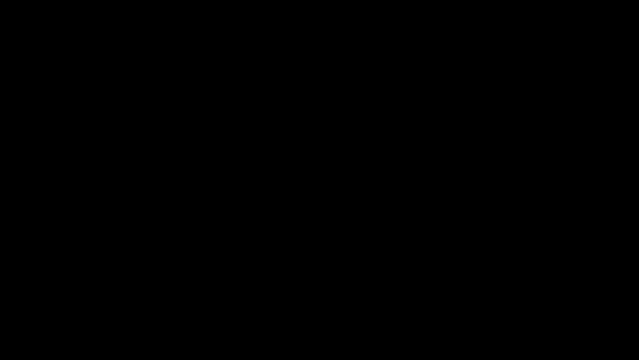 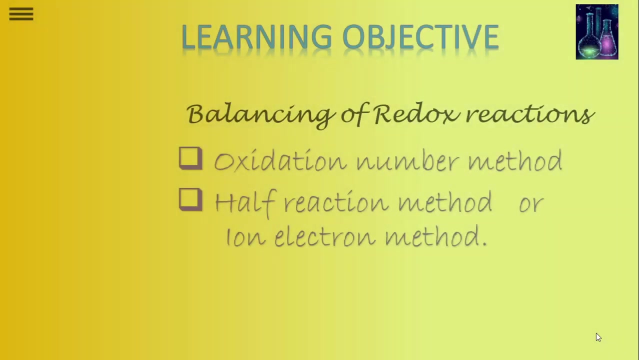 molecules of water will be cancelled out and finally I get my balanced equation. I hope you understood the oxidation number method and you can have the look on the steps once again. Now let's move on to our next method, that is, half reaction method or ion electron method. 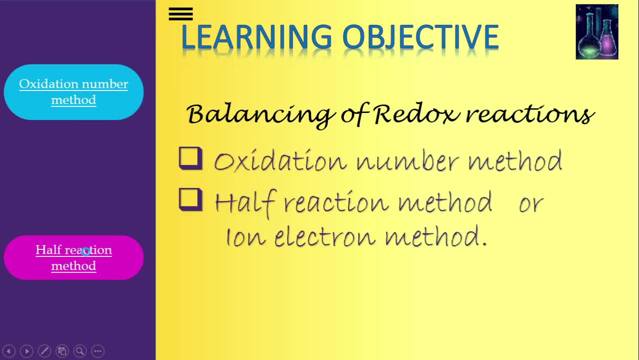 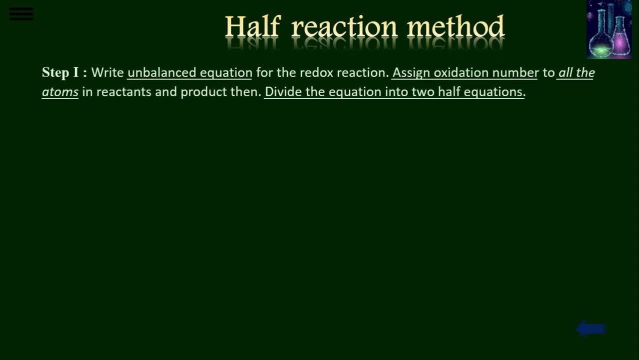 The steps involved in half reaction method or ion electron method are: write unbalanced equation for the redox reaction and assign oxidation number to all the atoms in the reactants and products. Then divide the equation into two half equations. Step 2: balance the half equation for 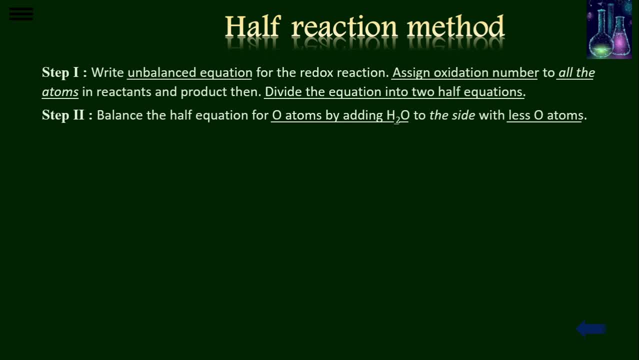 oxygen atom by adding water and then divide the equation into two half equations. Step 3: to the side with less oxygen atom: balance hydrogen atoms by adding H plus ions. to the side with less H plus ions. Step 4: balance the charges by adding appropriate number of electrons to 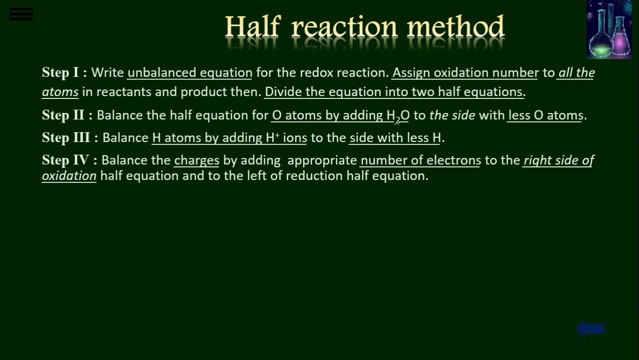 the right side of oxidation half reaction and to the left of reduction half reaction. Step 5''multiply half reaction' equation by a suitable factor to equalize the number of electrons in two half equations. Add the two half equations and cancel the number of electrons on both the side of the equation. 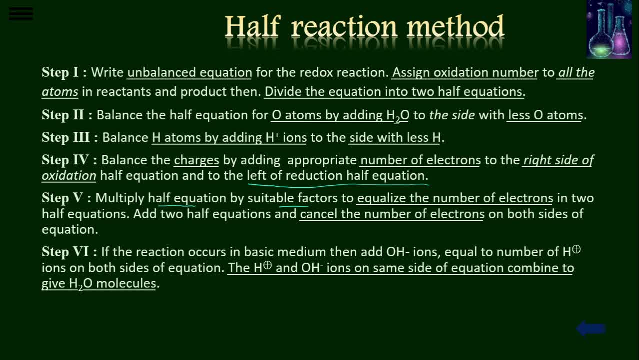 Step 6.. If the reaction occurs in basic medium, then add OH minus ions equal to the number of H plus ions on both the side of the equation. Then the H plus and OH ions are same side of the equation combined to give water molecule. And the last step, 7th step, check the equation. 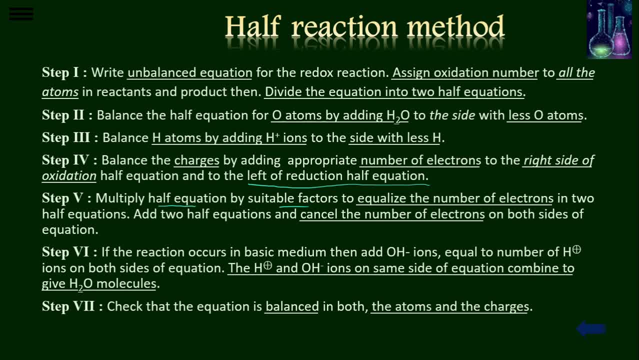 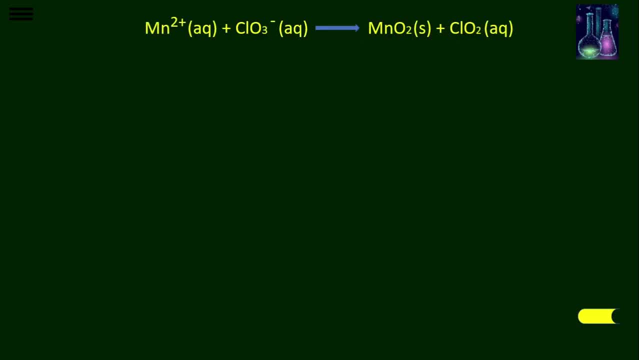 is balanced in both the atoms and the charges. Now let's apply the steps to some examples. The first example: Mn plus 2 plus ClO3 minus gives MnO2 plus ClO2.. So we have the skeletal equation in front of us. Now write the oxidation. 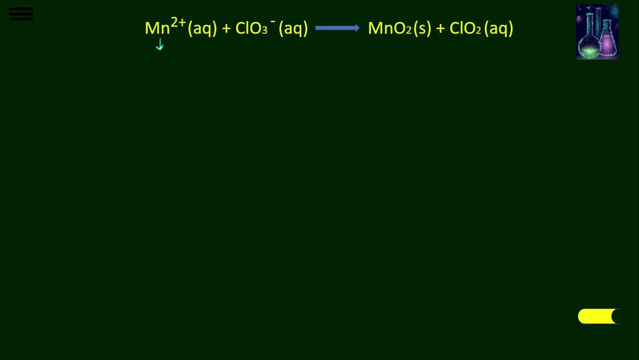 equation: Here Mn is plus 2.. Cl: here is plus 3. Oxygen: here is minus 2.. So this is our skeletal equation. Now let's assign the oxidation number: Here Mn is plus 2.. Here Cl is plus 5.. 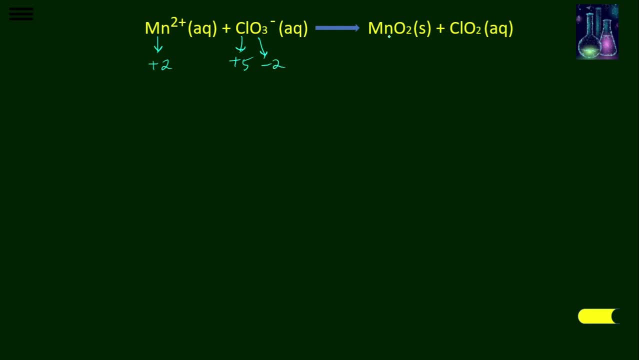 Oxygen here is minus 2.. Here Mn is plus 4.. Oxygen is minus 2.. Cl is plus 4.. And oxygen here is minus 2.. Now let's divide this equation into two half reactions. First let's write the oxidation half reaction: Mn plus 2 gives MnO2 plus ClO3 minus ClO2.. So this is our. 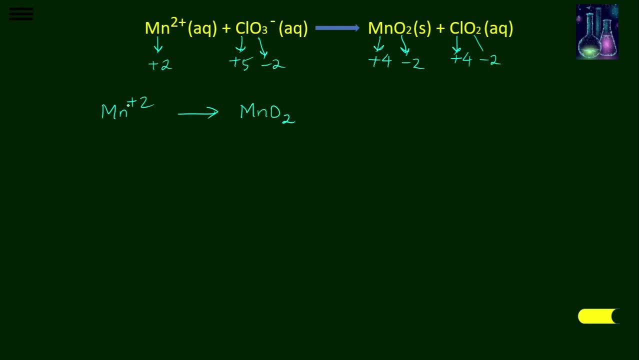 oxidation half reaction, Oxygen half reaction. That's why this is called as half reaction method, Oxygen half reaction. Now, when it changes from plus 2 to plus 4, it gives out two electron. That is oxidation Loss of electron. And 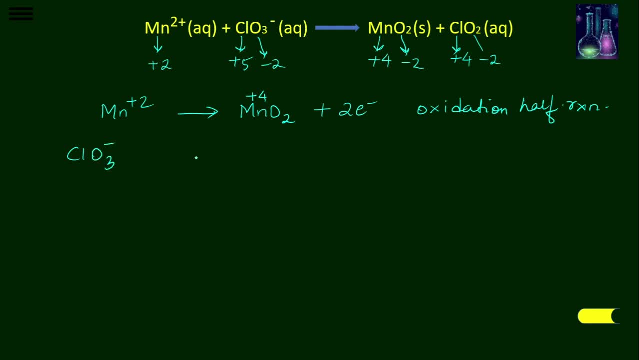 the oxidation number decreases. So this is reduction, half reaction. Now here the oxidation number decreases by one, So we have to put one electron. Okay, Now let's balance the oxygen atoms. Here you have one oxy, two oxygen, So I will put water. 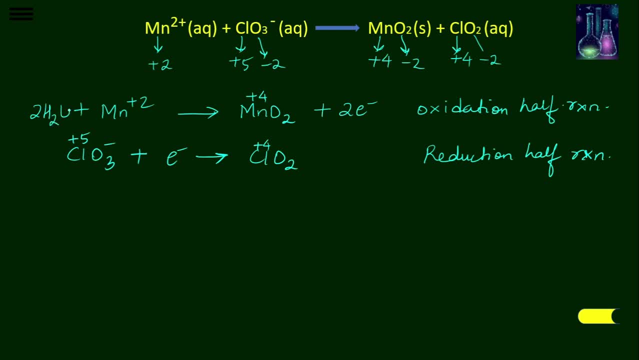 molecule, Two water molecules over here, And here I have three, And here I have two. So I have to add one water molecule above here. Now let's balance the charge. Here you have two electronsaff, Ok, one electron. so I'll multiply this by this by 2, so I'll have 2, 2, 2 and 2 now. 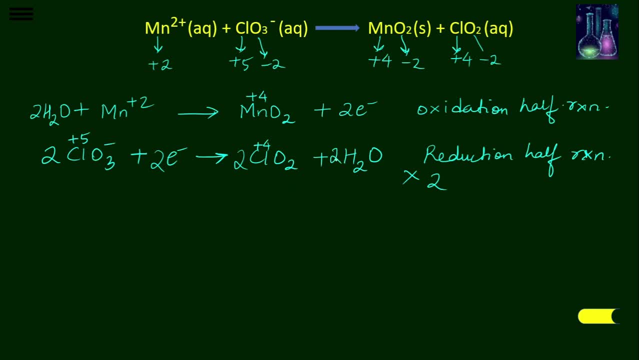 see for the H plus ions. here I have 4 H plus ions, 4 hydrogen atoms, and here I have 4 hydrogen atoms in the second reaction. so first I will add the hydrogen ions over here, 4 H plus ions, and here I will add 4 H plus ions. now 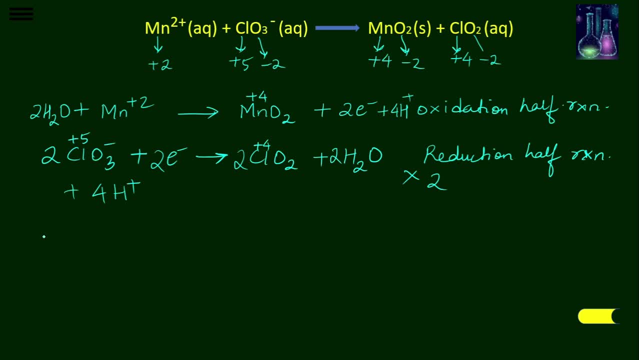 the two reactions are balanced. now just add them: 2H2O plus MN plus 2 plus 2Cl. 2ClO3- plus 2 electrons plus 4H plus gives MnO2 plus 2 electrons plus 4H plus plus 2ClO2 plus 2H2O. 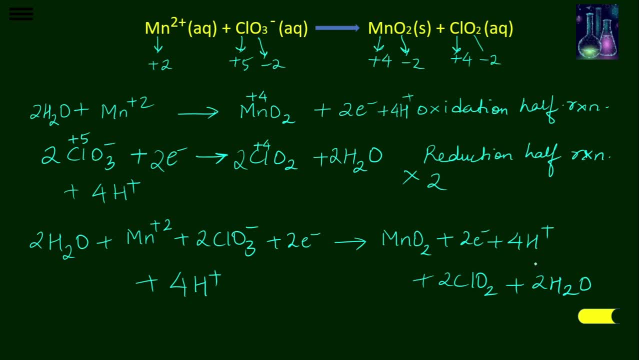 Now let's cancel what is common: 2 electron, 2 electron, 4H plus 4H plus 2 water, 2 water, and ultimately you get your balanced chemical reaction. that is Mn, that is Mn plus 2 plus 2ClO3-. 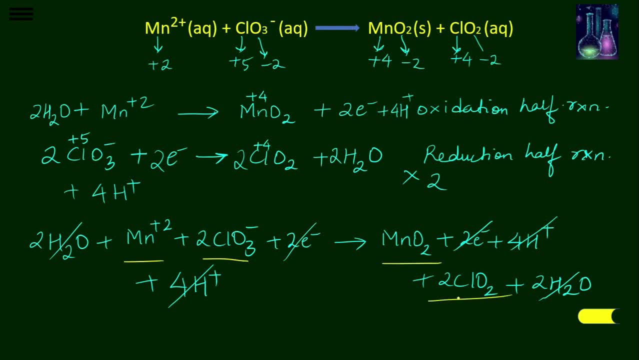 So this gives MnO2 plus 2ClO2 and I guess the charges are also balanced: here plus 2 charge, here minus 2 charge. here it is neutral and Mn, 1Mn, 2Cl, 2Cl 3, 2 is a 6 oxygen, here 2 plus 4, 6 oxygen. 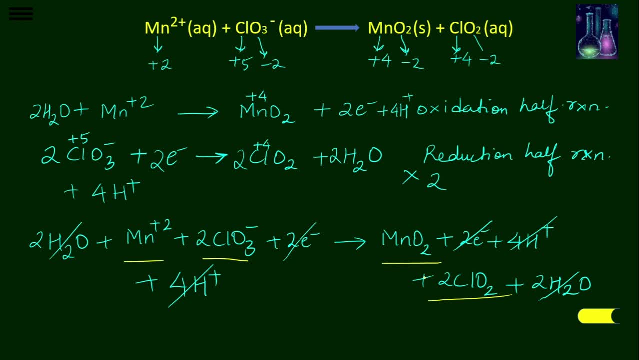 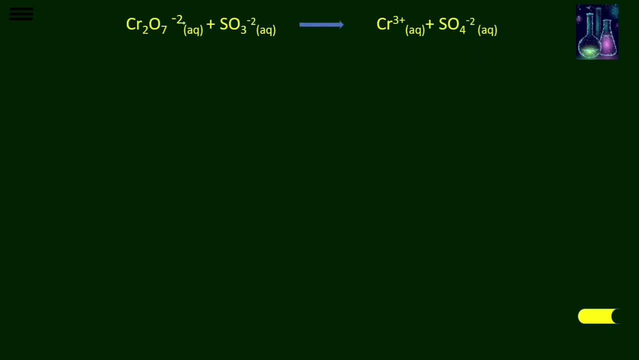 So ultimately you get your balanced chemical equation Easy. Let's move on to the next, Next example. 2Cl2O7-2 dichromate ion plus SO3-2 sulfate ion gives Cr plus 3 plus SO4-2 sulfate ion. 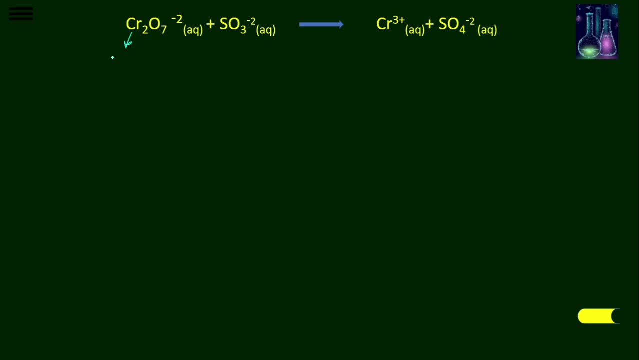 So let's assign the oxidation state Here: chromium is plus 6 each, oxygen is minus 2 each. sulfur: here is plus 4, oxygen minus 2.. Chromium here is plus 3, sulfur here is plus 6 and oxygen here is minus 2 each. 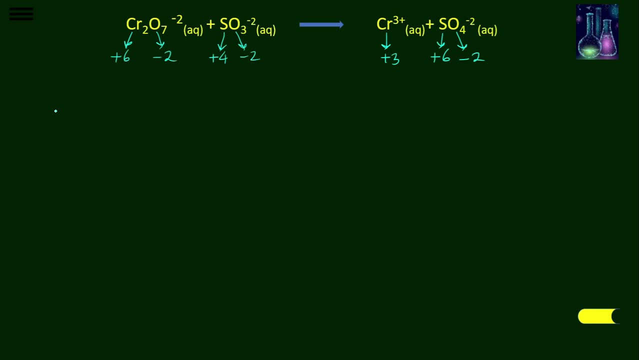 So let's write the oxidation half reaction. The oxidation half reaction: Here SO3-2 is converting into SO4-2.. So SO3-2.. So SO4-2.. So SO3-2. So. 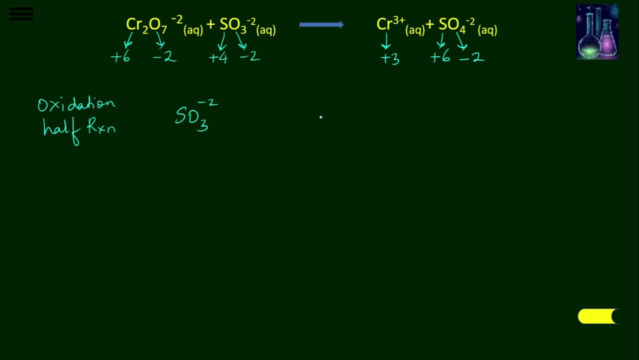 SO4-2.. So SO4-2.. SO3-2 converts into SO4-2 and reduction half reaction. the reduction half reaction is CR2O7, the whole minus 2 to CR plus 3.. Now, once we have identified the reduction half reaction and oxidation half reaction, let's now go on to the next step. 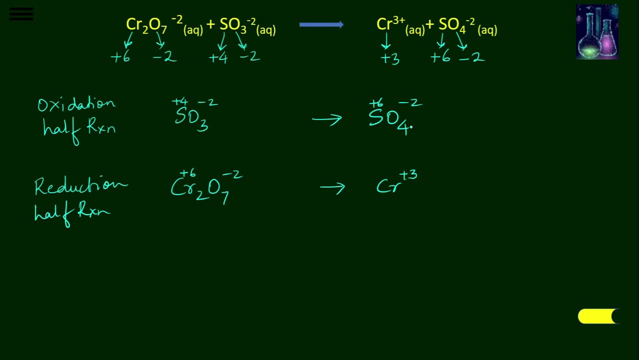 Balance the oxygen atom. Here you have 3 oxygen, here you have 4 oxygen. So we will balance it by adding a molecule of water, H2O, and here there are 7 oxygen atoms. So therefore, add 7 H2O to this. 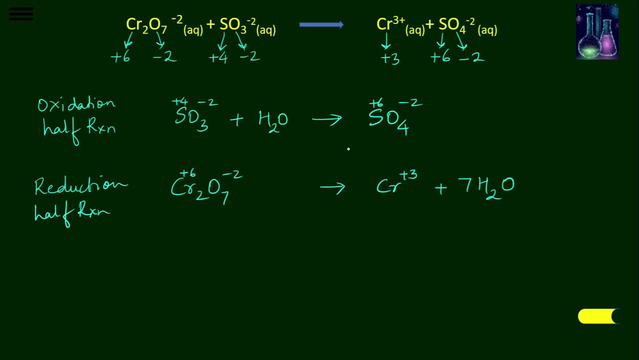 Next balance the hydrogen atoms. Here you have 2 hydrogen, so I will add here 2 H plus ions, and here I have 7 to the 14 hydrogen atoms, So I will add 14 H plus ions. Next balance the charges: From plus 4 it has gone to plus 6.. 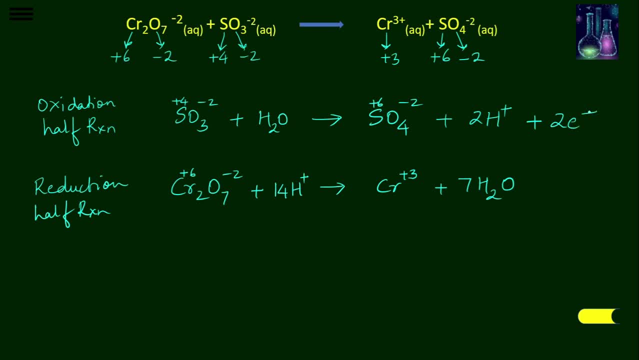 So it has undergone oxidation by loss of 2 electrons, and here it has converted From plus 6 to plus 3.. So it has gained 3 electrons. So here 3 electrons Now balance the chromium atoms as well. Here you have 2 chromium, here you have 1 chromium. add 2 chromium here. 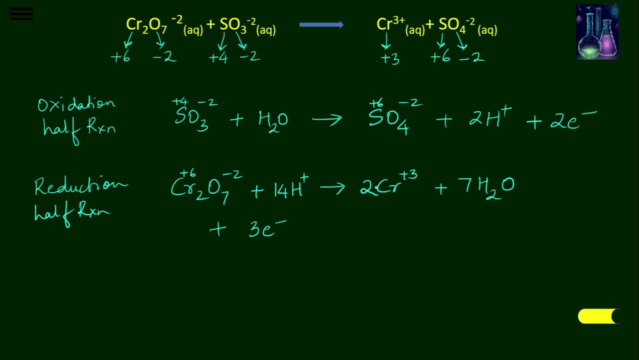 And since 1 chromium atom receives 3 electrons, so when you have 2 chromiums there will be 6 electrons. Now balance the electrons: Here you have 6, here you have 2.. So multiply this equation by 3.. 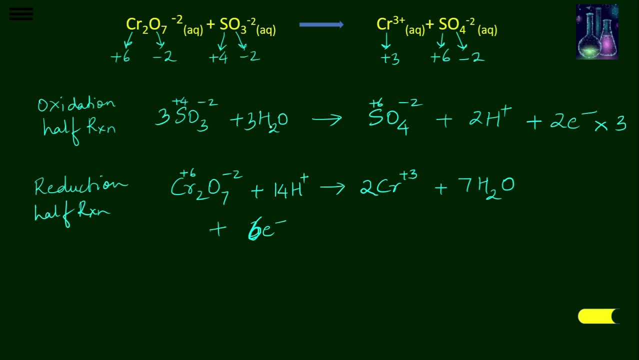 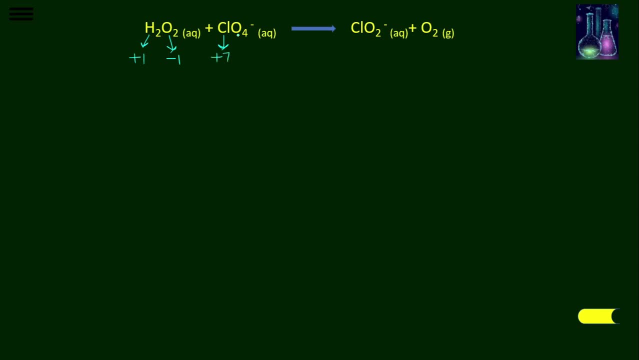 here oxygen is minus 2 H, here chlorine is plus 3 and here oxygen is minus 2 H and oxygen here is bonded to itself 3, so oxidation state is 0. now let's write the oxidation half reaction. so the oxidation half reaction is H2O2, gives O2. 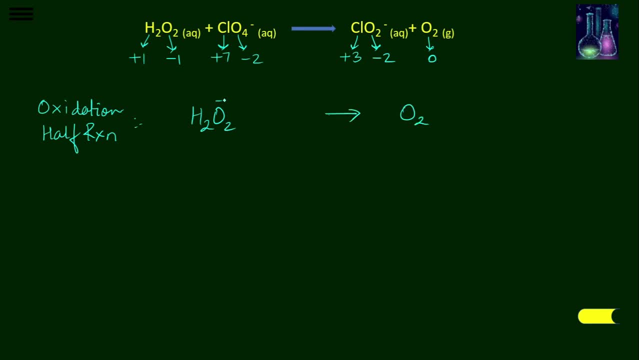 so minus 1 to 0, there is an increase in oxidation number. and next is the reduction half reaction. minus 1 to 0, there is an increase in oxidation number which can be written as ClO4 minus, converting into ClO2 minus. ok, now let's balance the hydrogen. 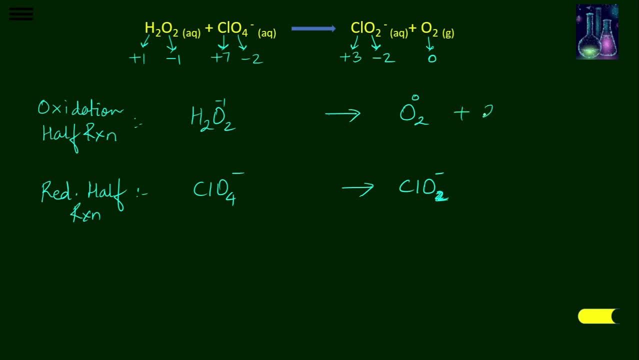 so here you have 2 hydrogen, so add 2 molecules of water. sorry, 2 H plus ions over here. so here you have 2 hydrogen, so add 2 molecules of water. and for oxygen, here there is 4 oxygen, here there is 2 oxygen. 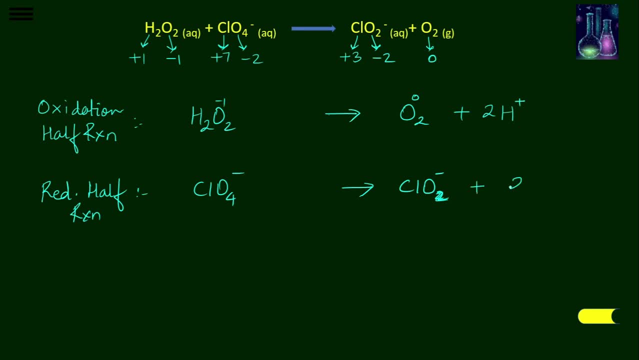 so add 2 molecules of water. on doing so you added 2 hydrogen, 4 hydrogen atoms as well. so I will balance that by adding 4 H plus ions over here. next, balance out the number of electrons. here I have lost electrons. so here plus 2 electrons, and here, from plus 7, I have reached to plus 3. 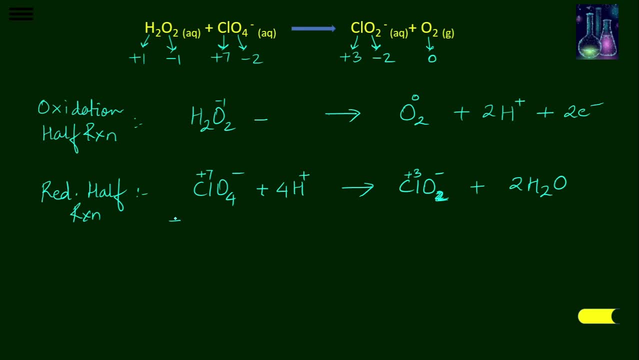 so here you will have 4 electrons. now, here there are 4 electrons, here there are 2 electrons. so multiply this equation by 2, so this makes up 4, sorry, 2 H2O, 2 H2O, 4 H2O, 2 H2O gives 2 H2O, 2 gives 4 H plus. 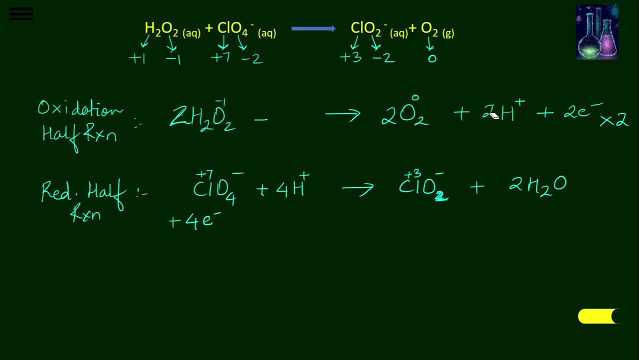 so this will now become, and this will also become 4, so here it will be 4 H plus ions, and here it will be 4 electrons. now see the balancing here. so here I am balancing: 2 hydrogen, 2 oxygen, 2 oxygen, 4 hydrogen and 4 electrons.